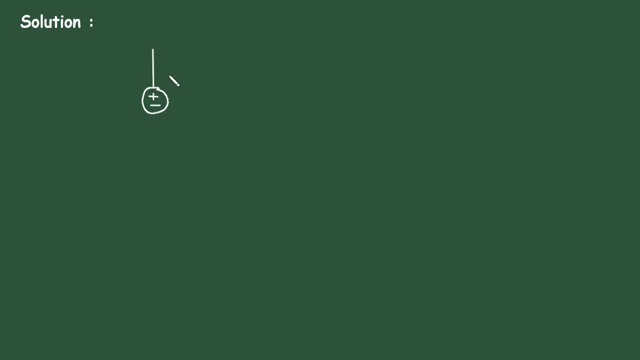 equivalent circuit, that is Thevenin voltage, in series with Thevenin's resistance. so this will be our Vth, that is Thevenin's voltage, and this will be our Rth, that is Thevenin's resistor. and here this will be our load resistor RL. this will be RL. this will be current IL. 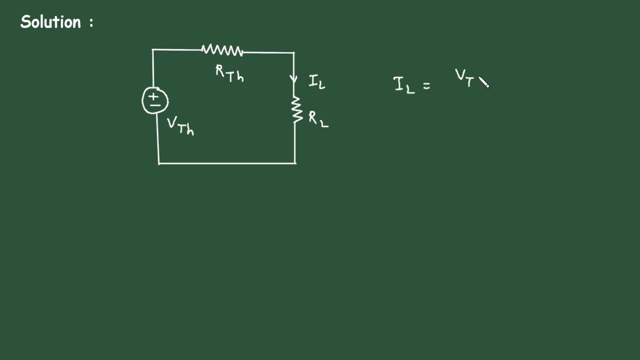 and current IL is equal to: can write. IL is equal to Vth upon Rth plus RL, Rth plus RL, And this will be our Thevenin's equivalent circuit. Now, first of all, to get this circuit here we will find the value. 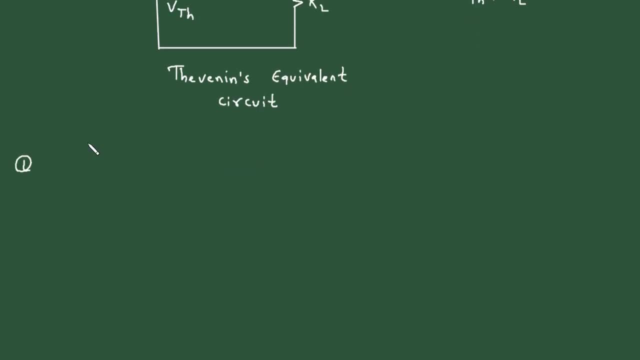 of Rth first. So step number one will be: find Rth, that is Thevenin's resistance. Now to find Rth. step will be: remove RL. remove RL and turn off all independent sources, independent sources. So here we will remove RL and this is our RL. that is this: four kilo ohm is the value. 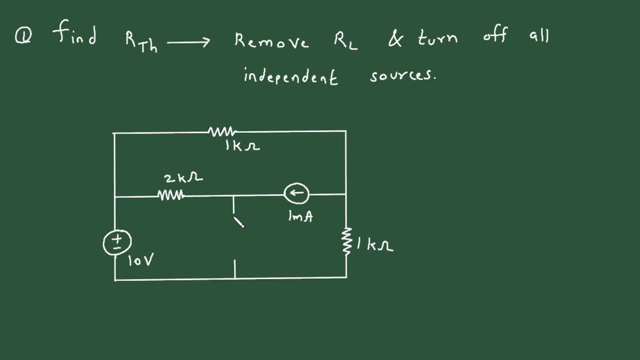 of RL. Let's say, this is terminal A and this is terminal B. Now, next thing we have to do, we have to turn off all the independent sources. So we will turn off this current source Now. when we turn off the current source, that time it will be a open circuit. 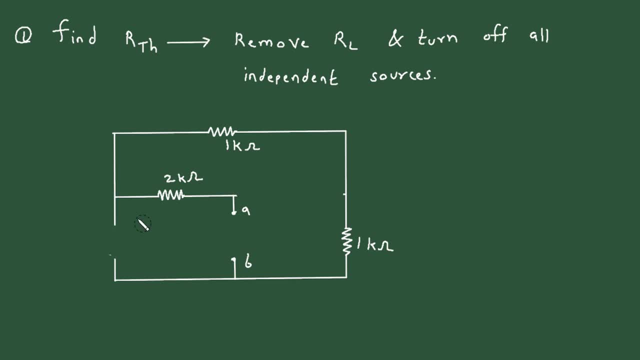 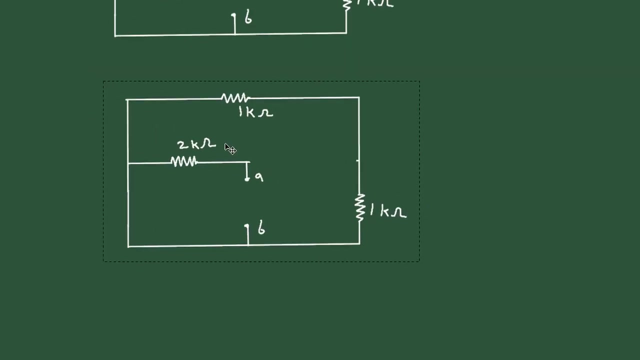 And when we turn off the voltage source, that time it will be a short circuit. we have to replace the independent sources by its internal resistance. Now, if we stretch this A and B, suppose if we stretch this A and B, then we will get the value of Rth Here. 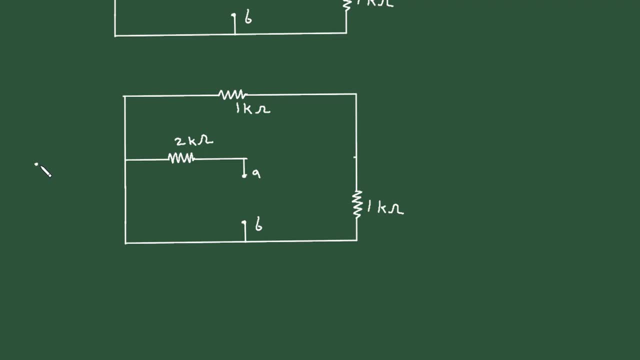 if we stretch this A, it will be like this: This will be our two kilo ohm And this is terminal A. Now next, if we stretch B- so let's say, this B will be here. We can stretch it like this: 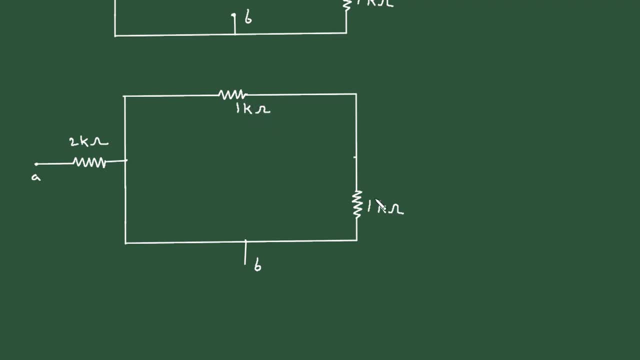 Now, this one kilo ohm and this one kilo ohm are in series, but they are short circuited, So here this will be zero. This is two kilo ohm, but it is short circuited, So that's why it will be zero. 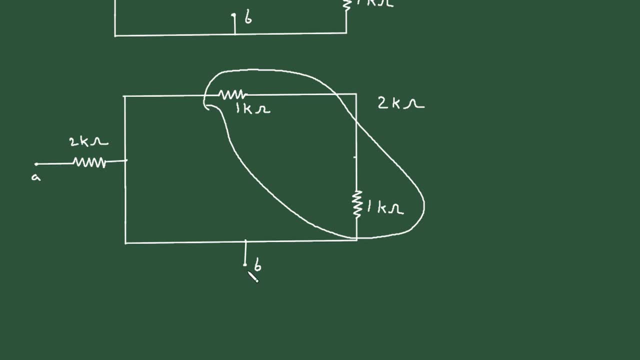 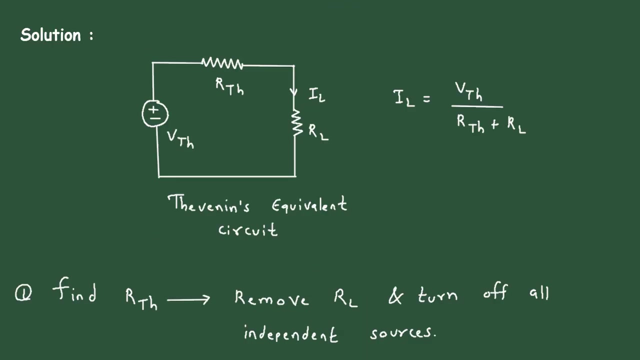 So therefore the resistance between A and B terminal will be only this: two kilo ohm. So therefore Rth is equal to two kilo ohm. Now we got the value of Rth. Next we have to find the value of. here we can see. we have to find the value of Vth, that is Thevenin's voltage. Next, 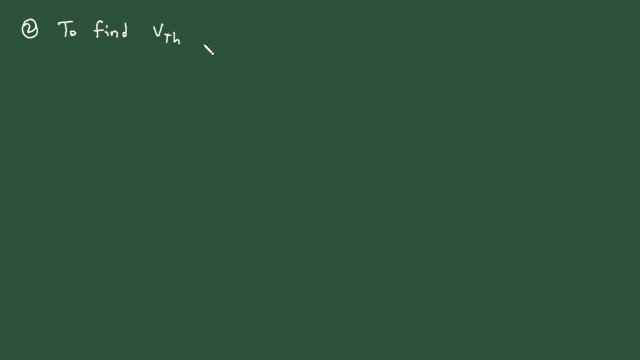 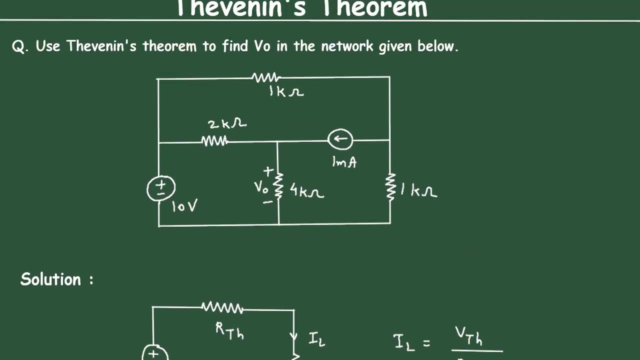 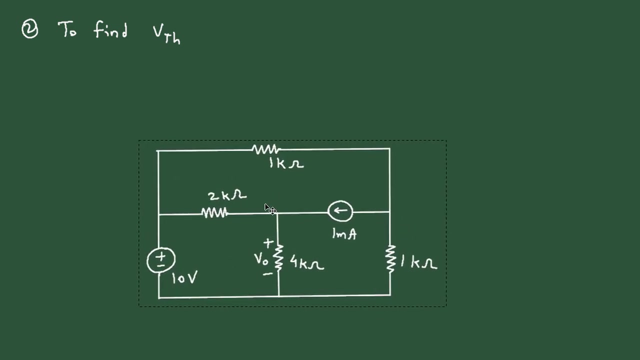 to find Vth. Now to find Vth Again, we will copy this circuit. first To find Vth again we will remove. to find Vth, remove RL. So first we will remove this RL And again this will be terminal A and this will be terminal B. 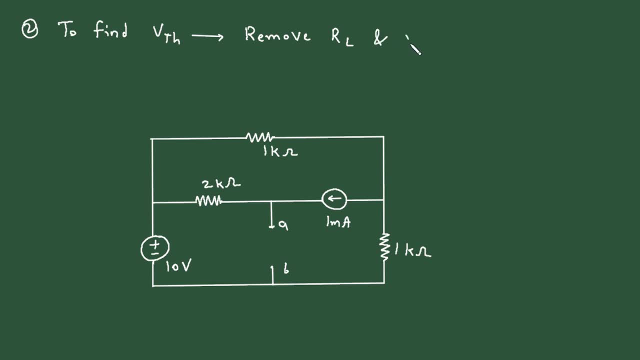 And next step will be: and voc is equal to Vth, So this will be our open circuit voltage voc. we will find the value of this voc. Now, to find the value of this voc, that is, this voltage. So here we can apply. Let's say we can. 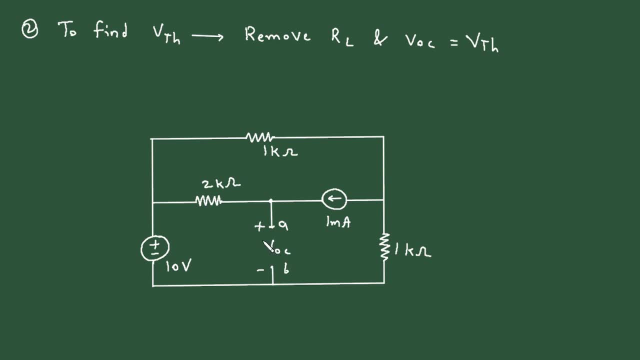 find it by using mesh analysis. let's say So. let's say this is mesh number one. We can see that this is mesh number one with current i1. And this is mesh number two. This will be mesh number two with current i2.. This is B. Now we will apply KVL to mesh number one, So apply. 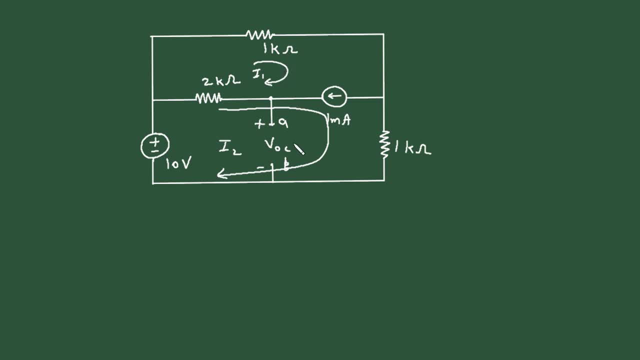 Here we can see, between mesh number one and mesh number two there is a current source, So this forms a supermesh. So this hole will be a supermesh. So first of all we will apply KVL to supermesh. So apply KVL, that is Kirchhoff's voltage law, to supermesh. Let's say we will start from. 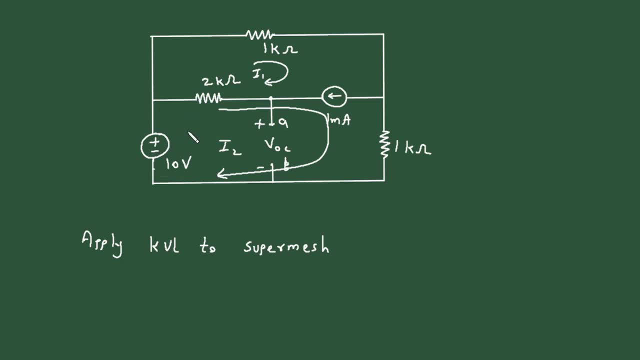 this point Now, according to the direction of this current, This will be positive, positive, this will be negative. this will be positive, this will be negative. so we will start from here. so it will be minus 10, then plus 1 kilo ohm, so 1 into 10, to the power 3 multiplied. 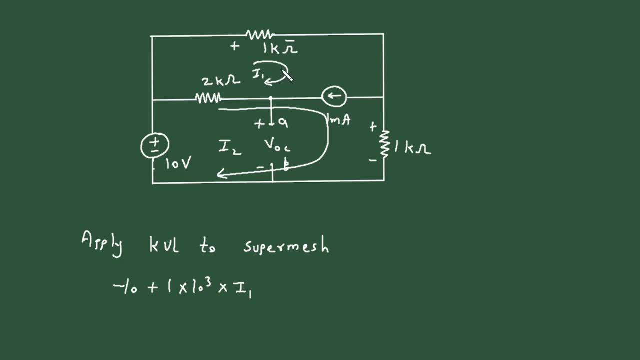 by current value is i1, then next is plus 1 kilo ohm. again 1 into 10 to the power 3 multiplied by i2 is equal to 0, so this will be 1, or directly we can write 10 to the power, 3 into i1 plus 10 to 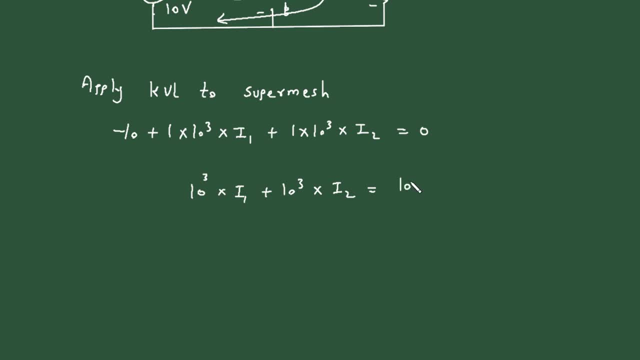 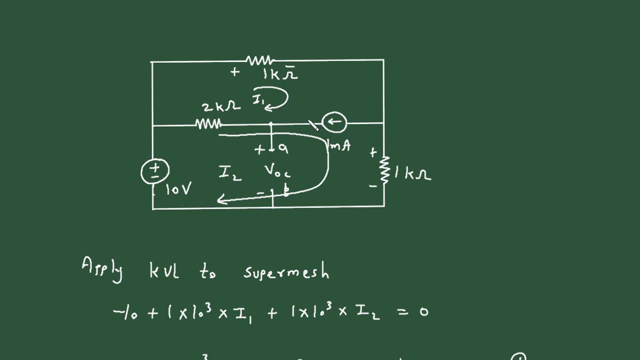 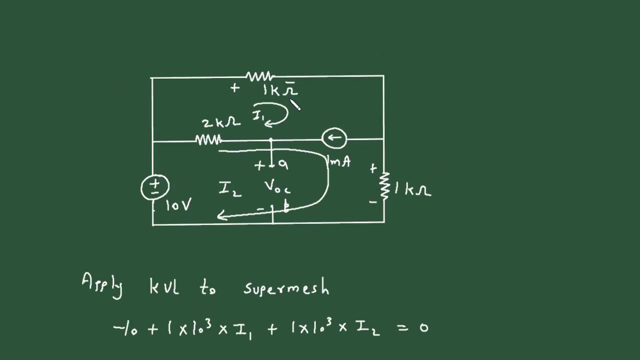 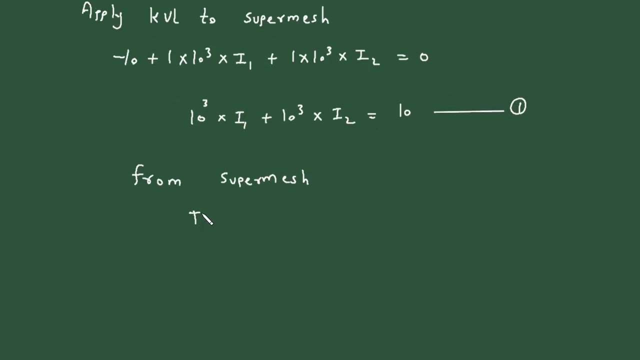 the power 3 into i2 is equal to 10. let's say, this is equation number 1. now next we will here. here we can see from super mesh again we can say so from super mesh: i1 minus i2 is equal to 1 milliampere. i1 minus i2 is equal to 1 milliampere. that is, 1 into 10 to. 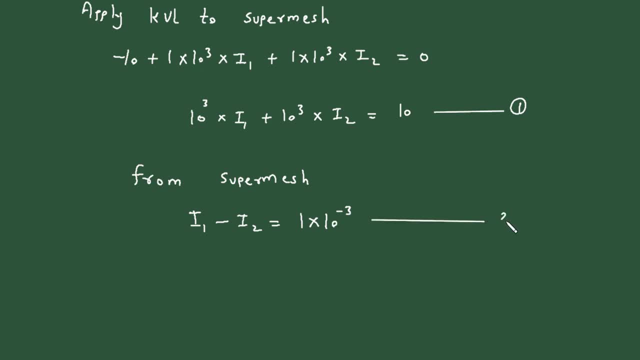 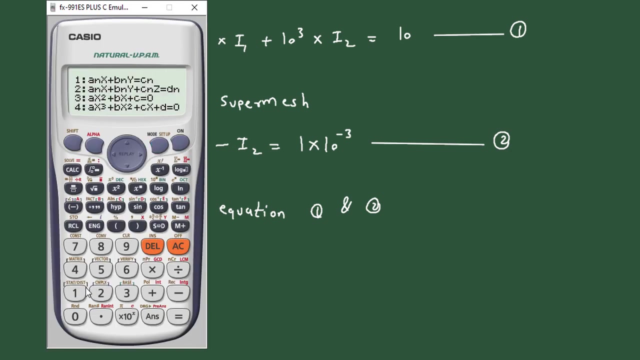 the power minus 3. let's say this is equation number 2. now we will solve equation number 1 and 2. so solve, solve, solve, solving equation one and two. So if we solve equation one and two we get the value of i1 and i2.. So in calculator there are two unknowns, So pi? u and one. Now this will be. 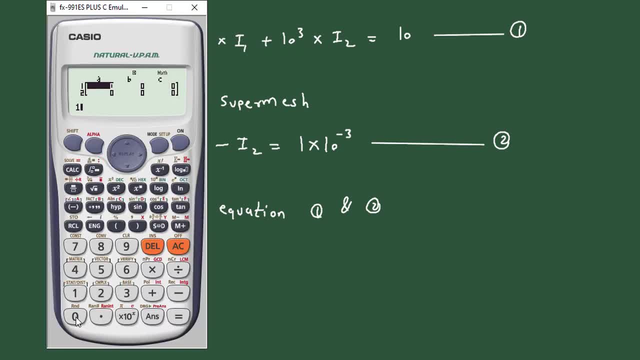 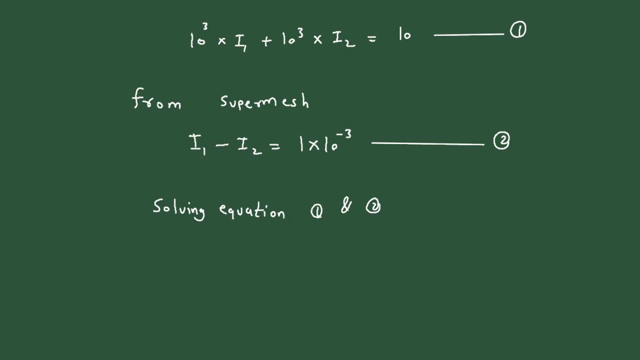 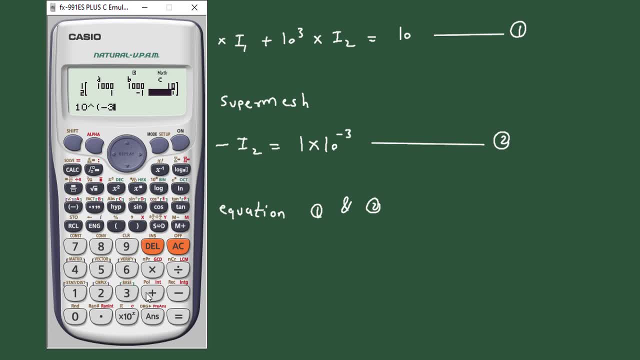 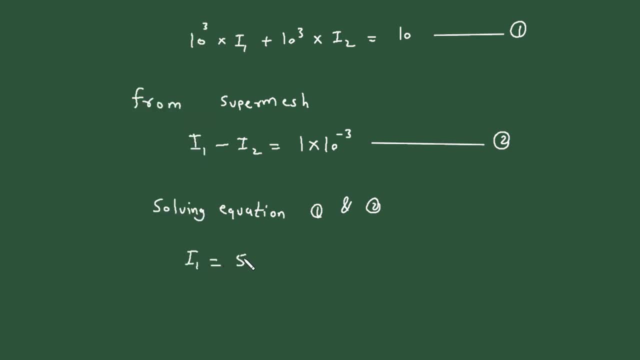 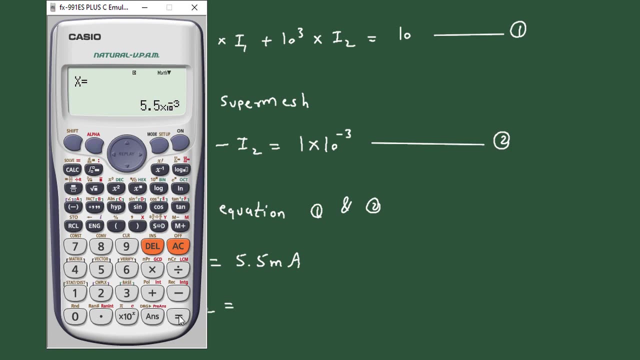 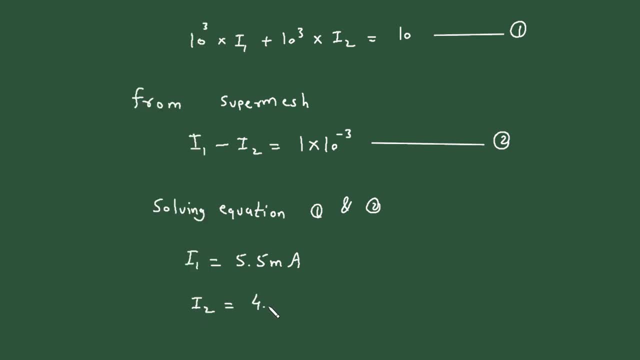 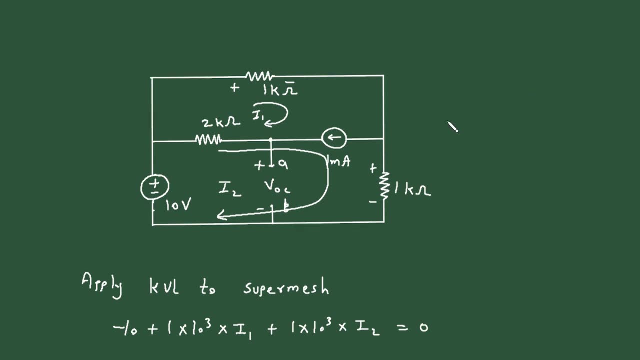 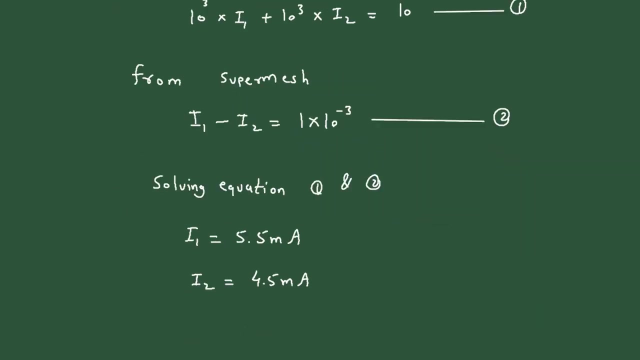 i1 is equal to 4.5 milliampere, 4.5 milliampere. Now we have the value of i1 and i2.. So we can find the value of this voc Again. we will copy this circuit here And let's say: this is loop. 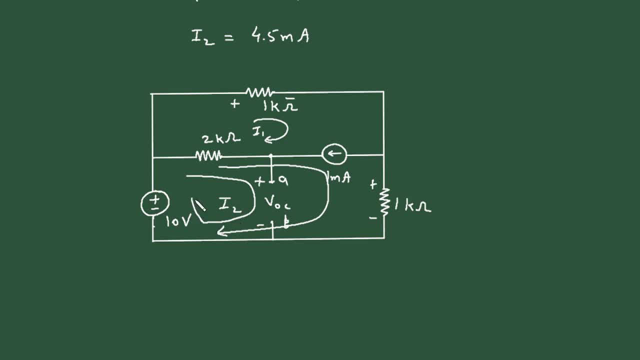 number three. This is loop number three with current i3. Now apply KVL, apply KVL to mesh. number three: Now here, according to the direction of this current i3, this will be positive, this will be negative And let's say, we will start from. 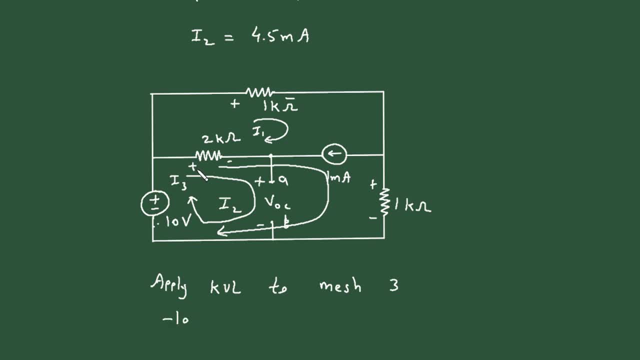 this point. So it will be minus 10, then plus, then this will be 2 kilo ohm, So 2 into 10 to the power 3.. in bracket i2 minus i1, so i2 minus i1, then plus voc, plus voc is equal to 0. now we have the value of. 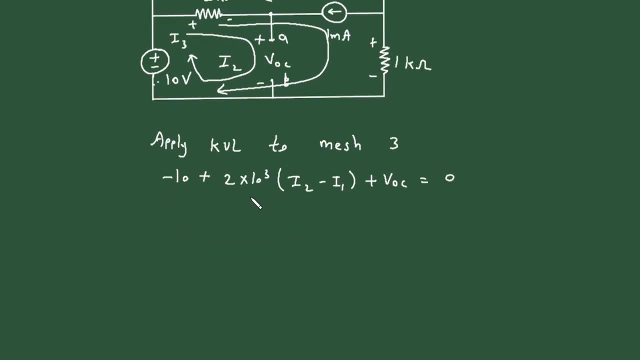 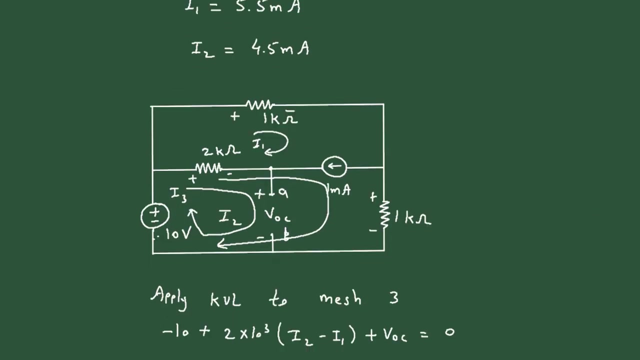 i2 and i1, so here we will substitute it. before that we will take it on right side. so voc is equal to: this will be 10, this will be minus 2, 10 to 10 to the power 3 in bracket i2, 4.5 milliampere. 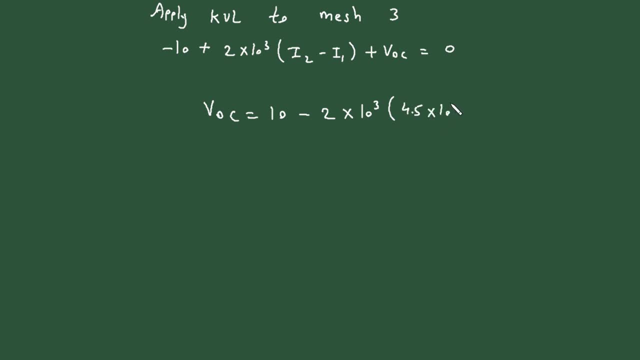 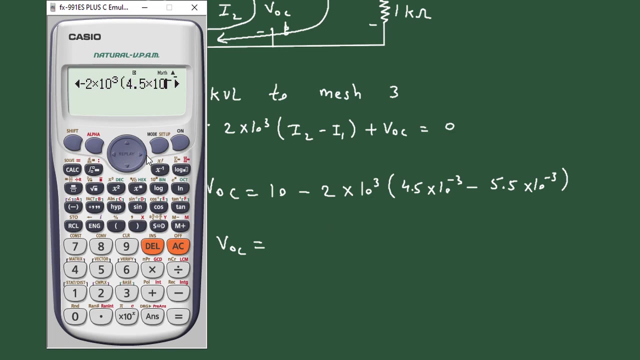 so 4.5 multiplied by 10 to the power minus 3 minus 5.5 milliampere. so 5.5 multiplied by 10 to the power minus 3. now if we solve this we get voc is equal to 10 minus 2 into 10 to the power, 3, 4.5 into 10 to the power minus 3 minus 5.5 into 10 to the power. 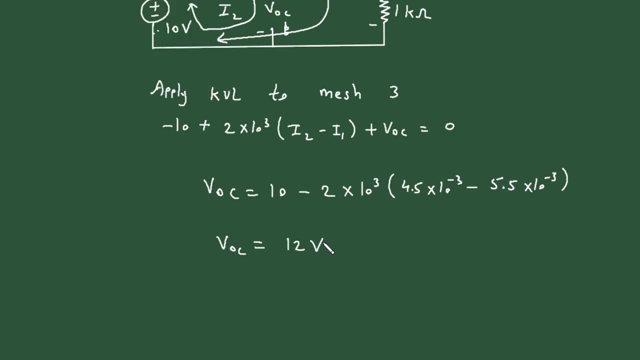 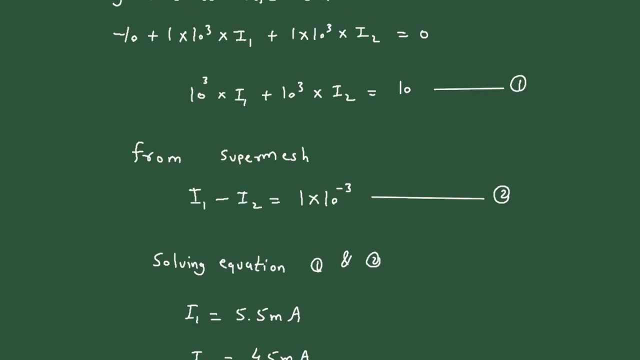 minus 3, it is equal to 12. so it is equal to 12 volt. this is the value of voc, and voc is equal to vth. so therefore, vth is equal to 12 volt. now we have the value of vth, vth and we have the value of. 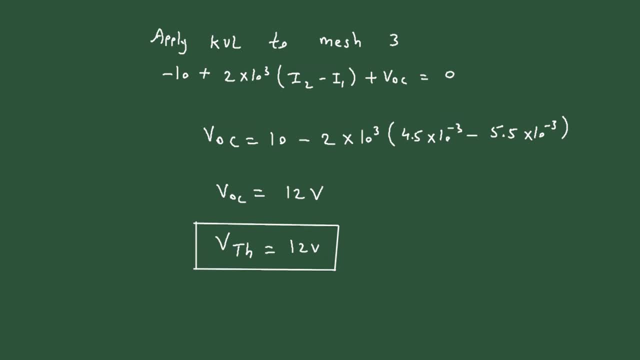 voc and vth. now we can draw thevenin equivalent circuit from thevenin's resistance and thevenin's voltage. so its equivalent thevenin's circuit will be: this will be rth, this will be vth. vth is equal to 12.5 milliampere. 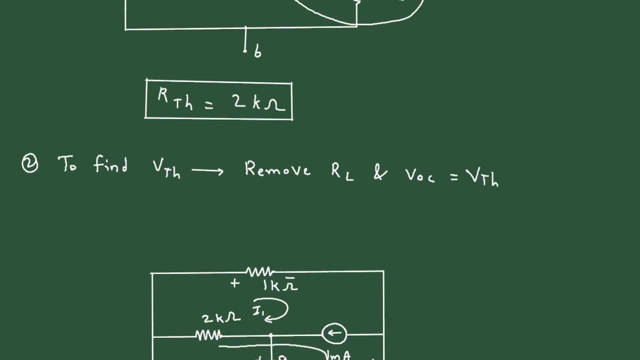 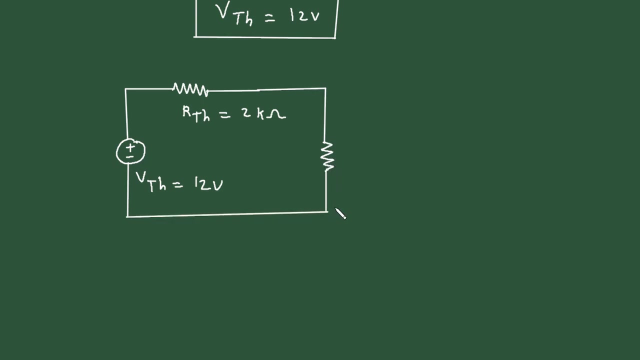 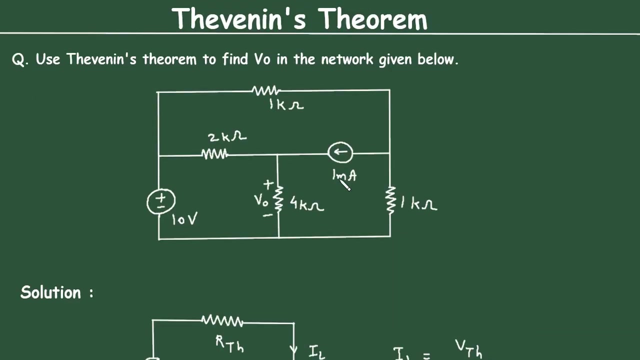 volt and rth is equal to 2 kilo ohm. 2 kilo ohm and this is our rl. the value of rl is: this is our rl. the value of rl is here. we can see: it is 4 kilo ohm. so 4 kilo ohm. 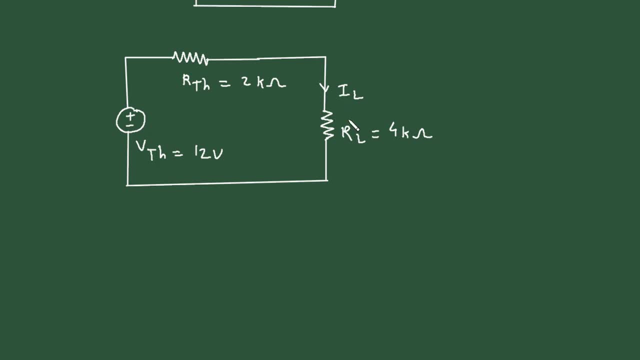 this will be current il. first we will find the value of il. here we can write: it is thevenin's, thevenin's equivalent, thevenin's equivalent circuit. so if we apply current division rule here, no need to apply current division rule here. uh, here we can directly find the value of il.